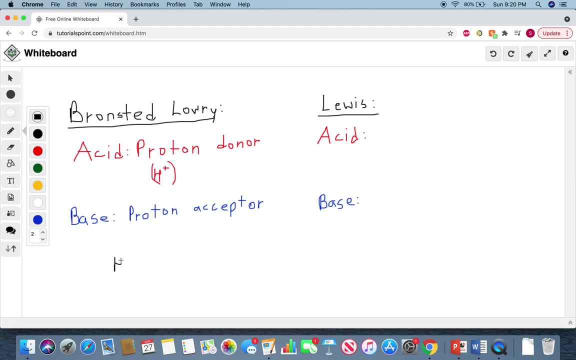 So let's look at an example. So let's say we have HCl or hydrochloric acid reacting with water And that gives us H3O plus or a hydronium ion plus a Cl minus a chloride anion. All right, so let's track what's happening here. So first thing that you should notice is that 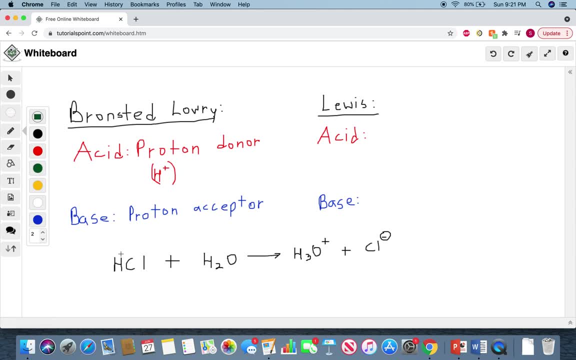 there is a transfer of this hydrogen ion from the HCl onto the water, And that's what makes H3O plus. So this chlorine no longer has that hydrogen, And because of that since. so the HCl is where the hydrogen is being donated from. So therefore, that by our Bronsted 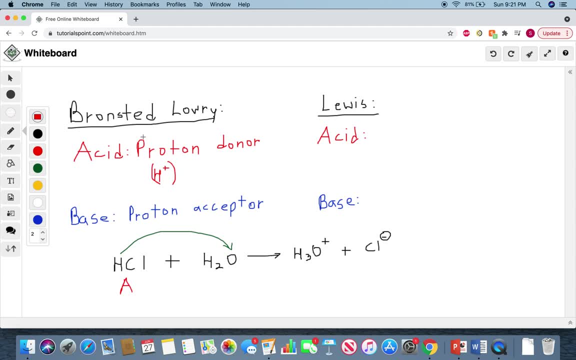 Lowry definition is our acid. All right, so that is our Bronsted-Lowry acid And, in that same definition, since water is the one that is accepting our proton, our H plus ion, it is our base. Okay, and then another thing, and more terminology that we also need to be aware of. 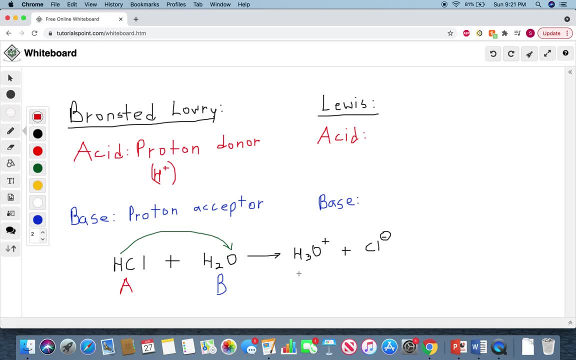 is that on the right side of our formula here we also have what is called our conjugate acid And our conjugate base. So how we determine those is our conjugate acid is basically again what our base becomes right So. but once our base receives the hydrogen or accepts the 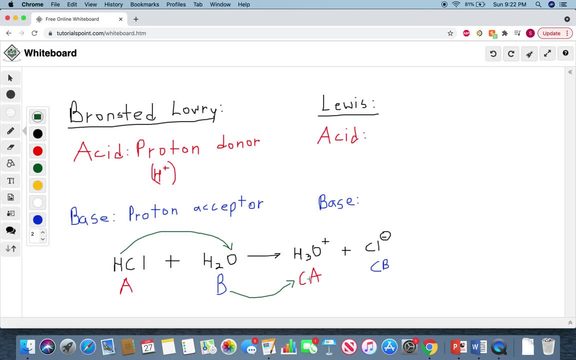 H plus or proton, it becomes the conjugate acid. And the same thing is with the same thing with the acid. So once the acid donates its hydrogen or donates its proton, it becomes the conjugate base. Okay, so that is the, that is using the definition of the Bronsted-Lowry acid and base. 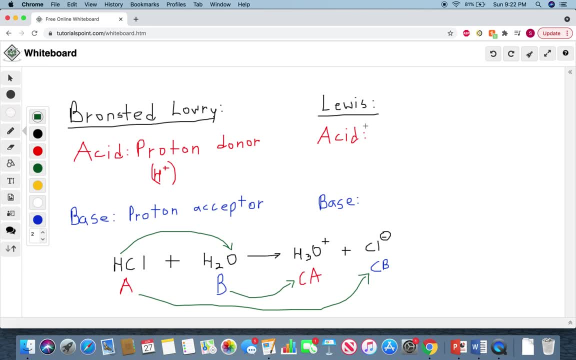 So let's compare that to the definition using Lewis acids and acids and base right. So with a Lewis acid, Lewis acid is described as an electron, So an electron pair acceptor. Okay, so an electron pair acceptor. So instead of defining it as a proton donor, we define it as accepting an electron pair And we 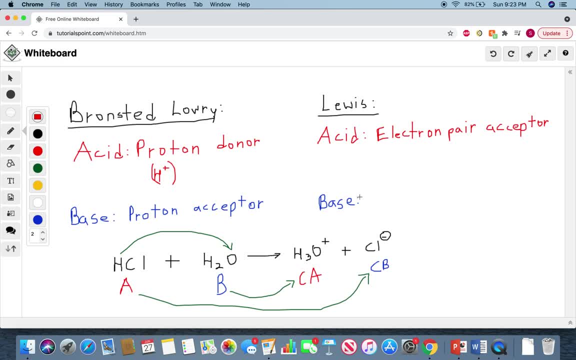 will be looking at examples of how we can see that, Whereas a base in as a Lewis base is defined as an electron pair donor, So electron pair donor. So, if you notice, the words donor and acceptor have been swapped between Bronsted-Lowry and Lewis. 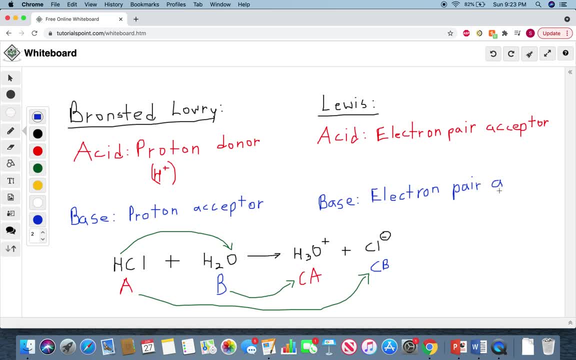 acid and base definitions. However, what we're donating and what we are accepting is very different. Okay, so keep track of that, because these definitions are extremely important. So, Bronsted-Lowry acid and base, Well, I something that you might have learned already before in general chemistry, but a Lewis 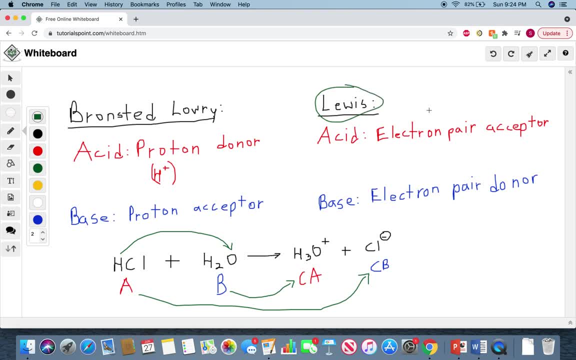 acid and base is the main focus of organic chemistry. Okay, so a lot. organic chemistry focuses mainly on the definition of Lewis acids and bases. Another thing that you should also be aware of is a Lewis acid is also called an electrophile. Okay, an electrophile. 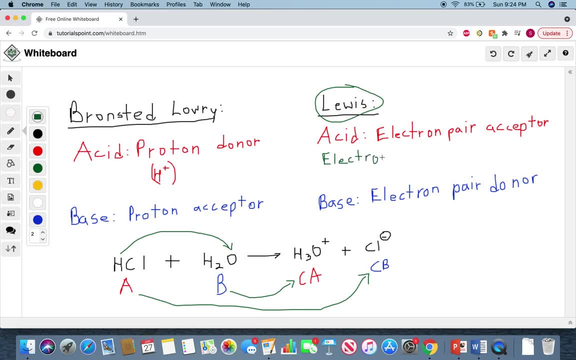 is also a Lewis acid. Lewis acid is also an electrophile. therefore, a Lewis base is also a nucleophile, So a Lewis base is also a nucleophile. So let's expand on these definitions. So let's talk about why we define them as this. 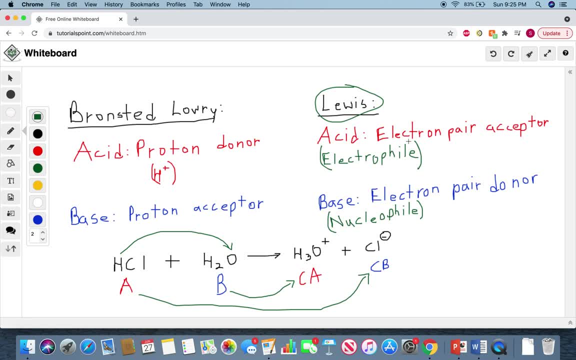 So a Lewis acid is defined as an electron pair acceptor. so what is happening? So it accepts an electron pair. Electrophile means electron loving, so it likes electrons, so it wants to take in electron pairs, Whereas a nucleophile is something that donates electrons. 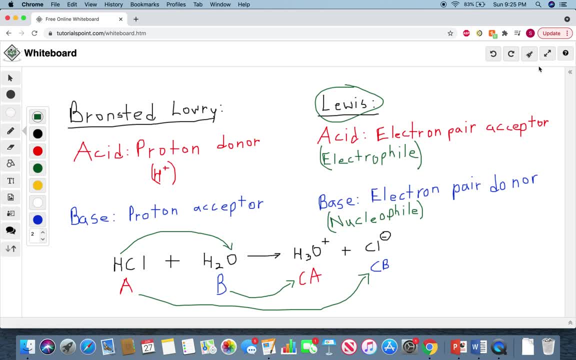 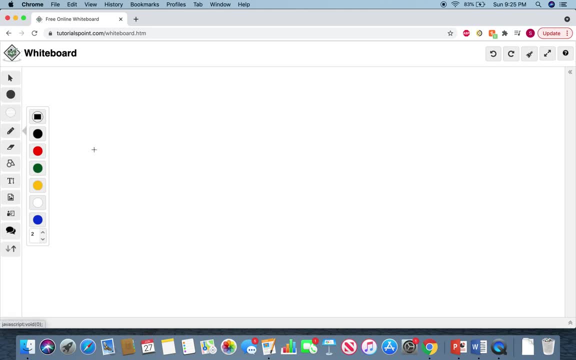 So let's look at that definition in this same example. So let's look at that. So let's say we have again we look at the HCl- a hydrogen that is bonded to a chlorine. correct, That's HCl And we are bonding that to a water. 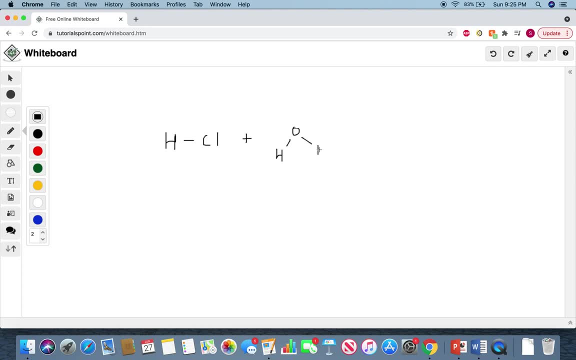 So it's an oxygen that has two hydrogens. That is our water. If we were to take this molecule, what is essentially happening is that this water, this oxygen of this water, is actually using its electrons right here, using its electron pair, to bond to this hydrogen, here And then. 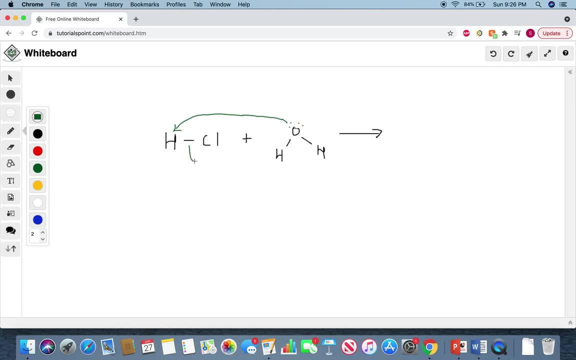 as it's bonding to this hydrogen. this hydrogen breaks off from this chlorine and the bond between the hydrogen and chlorine returns the electrons to this chlorine, And that is how we end up with this hydronium ion, This hydronium ion. 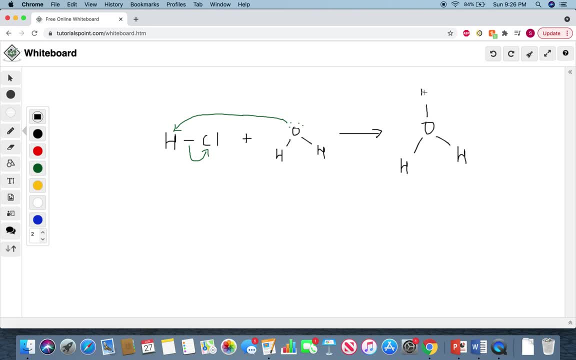 comes about because this oxygen bonds to this third hydrogen And we also end up with this chloride anion. So a chlorine that normally would have had just three lone pairs now gets a fourth lone pair from that bond that broke between the hydrogen and the chlorine. 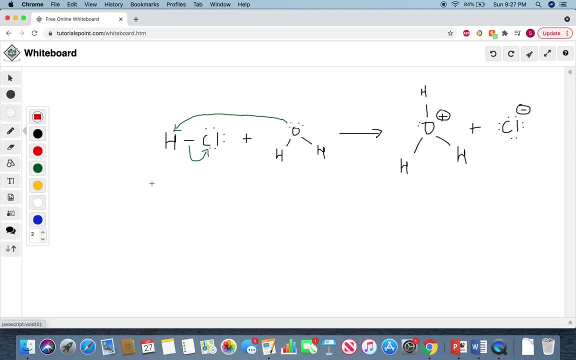 So what you should notice is that this, right here, what we described as an acid in our Bronsted-Lowry definition is still an acid in our Lewis acid definition, All right, and this is still our base in our Lewis acids and base definition. 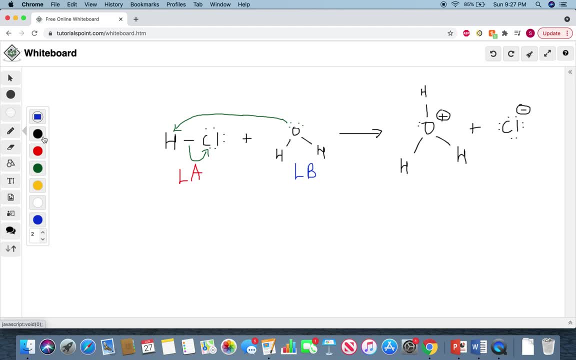 Okay, so that's something that you should notice. So what an acid is still remains the same, regardless of whether it's defined through the Bronsted-Lowry acid definition or the Lewis acid base definition. But it's just, we look at it differently, right. 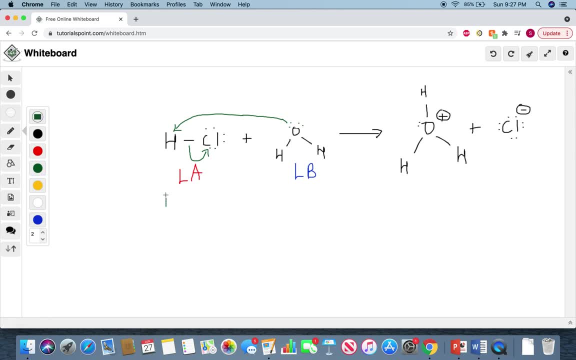 So the other thing that you should notice is that this right here is also our electrophile, and our electrophile is electron loving, so it gains electrons, right. so another thing that you should understand about these arrows is that the direction that the arrow points is where the electrons 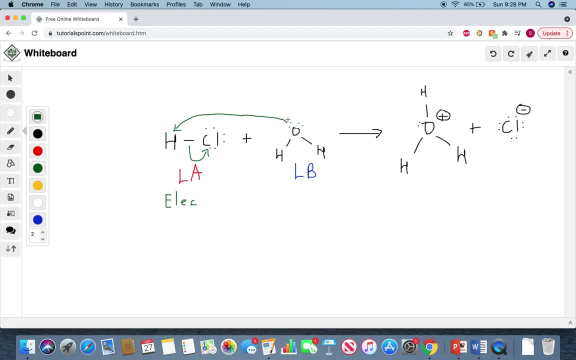 are going towards. alright, so that where it points from is the source of the electrons. where it points to is where the electrons end up. alright. so if you notice, with our chlorine or our HCl, right here the arrows are being pointed to the hydrogen and to the chlorine. so that is our electrophile, because that is. 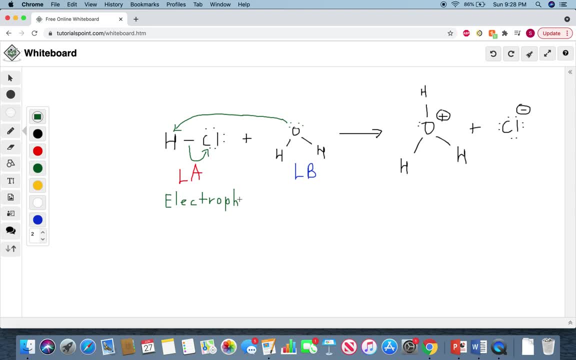 where the arrows are pointing to. that means that that's where the electrons are going towards and it's electron loving, so it's taking in those electrons, whereas our Lewis base, that's where the electrons are originating from, which is our Lewis base, and that, therefore, that is our nucleophile. so a nucleophile is where electron pairs. 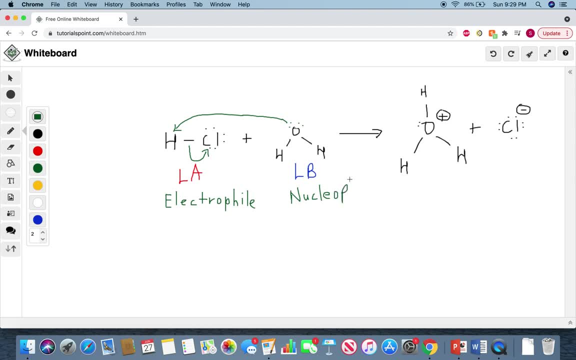 originate from. okay, so we will go into more detail about a nucleophile versus an electrophile later, but that is just a general definition of a Bronsted-Lowry acid and base versus a Lewis acid and base and how you would distinguish between them. okay, so, whereas in a Bronsted-Lowry acid and base, you would. 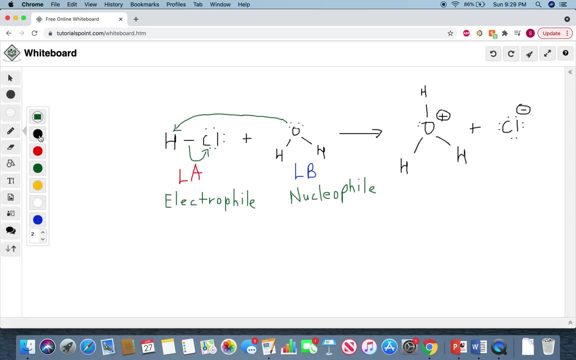 just directly look at. you would just directly look at. oh, we have a hydrogen here that was originally with, bonded to chlorine, but now it's been being donated to this water to give us our hydronium. so, therefore, that that would be our acid, because it's our 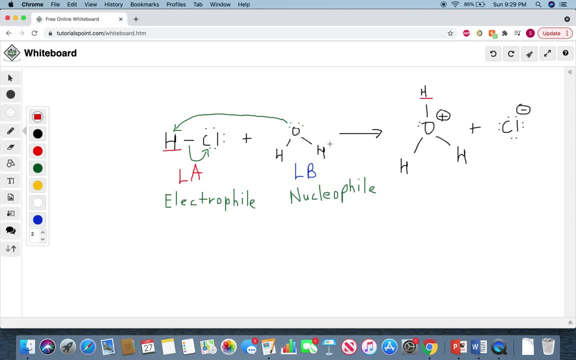 proton donor. therefore the other molecule would be our proton acceptor. so therefore our base, but with Lewis acid and base definition, we're just looking at it through a different definition right, which is through the electron, so with the acid being the electron pair acceptor with and where the base is the 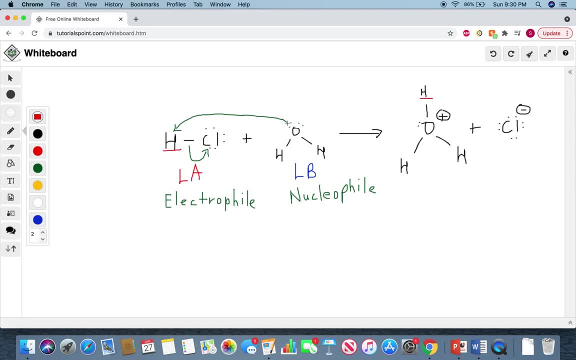 electron pair donor. and so again, the electron pair donor is where the arrow originates and the electron pair acceptor is where the arrow ends up being pointing to again. if you have any questions, go ahead and put them down in the comments again. I'm just starting this channel, so if there are other